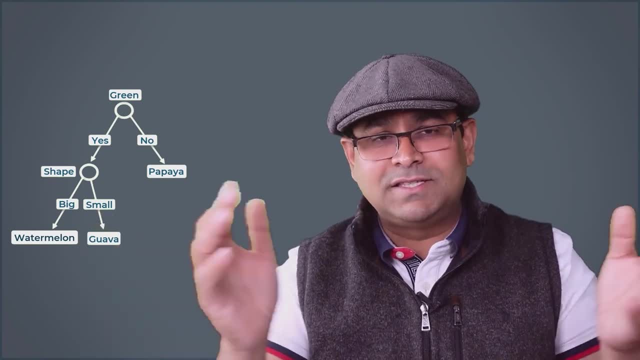 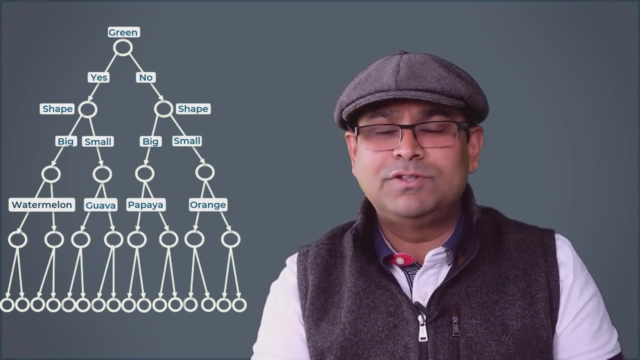 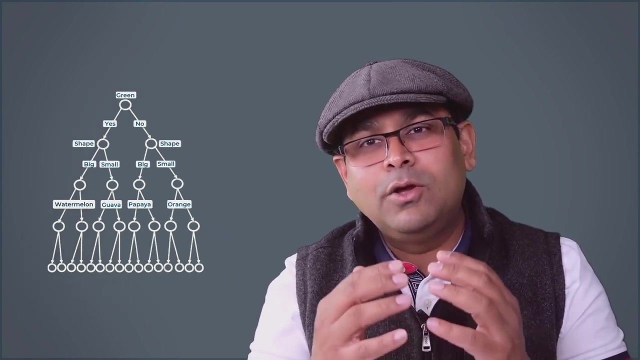 If you find this, do something. If you find that, do something else. Soon, the number of rules became overwhelming for even moderately complex tasks. It was very difficult to put these rules together, So researchers started asking what if the machines could learn by looking at data instead of trying to be programmed explicitly with rules. 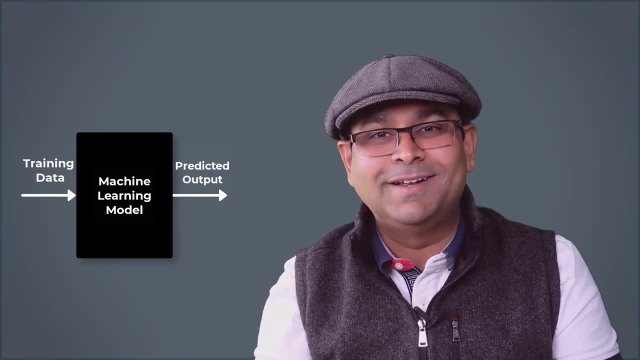 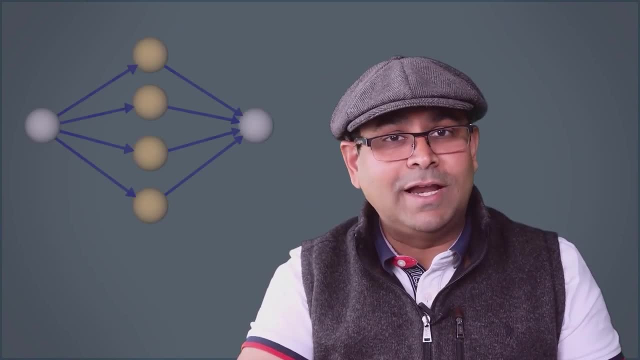 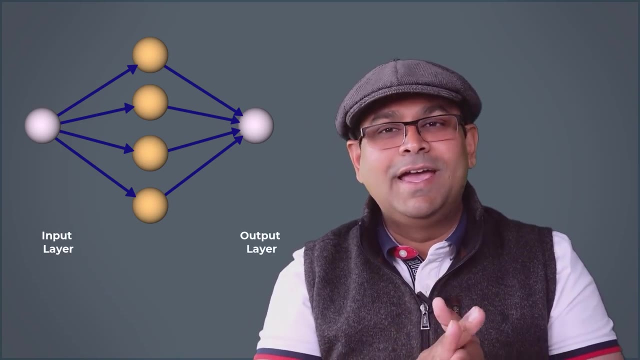 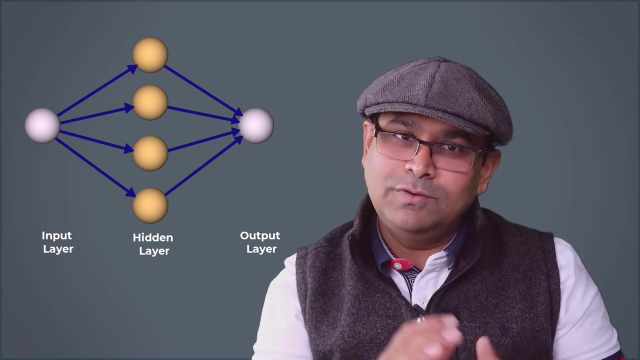 machine learning algorithms, and some of them are based on neural networks. Early neural networks contained three layers: an input layer for receiving input, an output layer and a third hidden layer. These neural networks could solve simple problems, but the media and some overly. 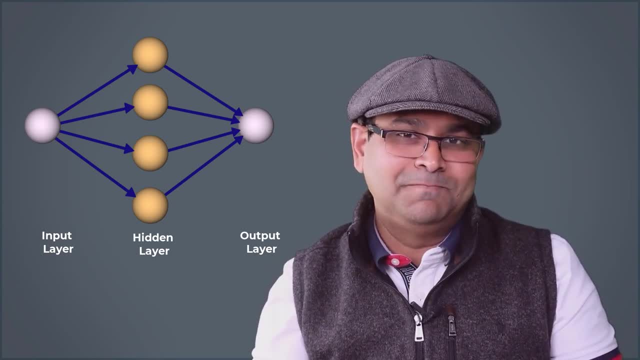 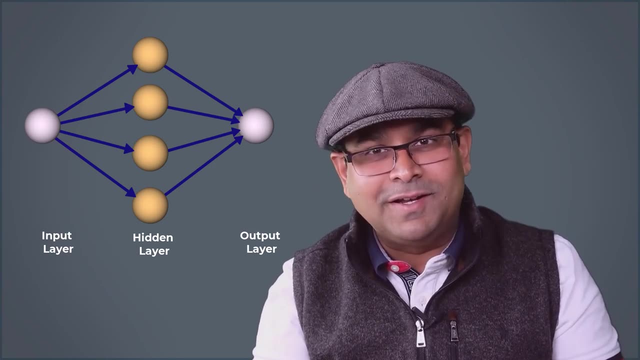 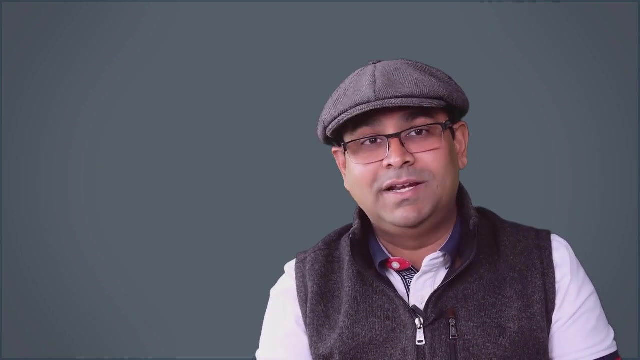 optimistic researchers hyped up their capabilities, So obviously these networks did not live up to their lofty expectations and there was a lot of disappointment and neural networks became a dirty word in AI. However, people working in the field were making good progress, They discovered. 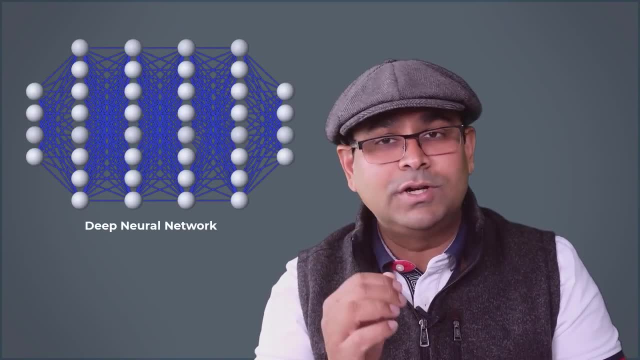 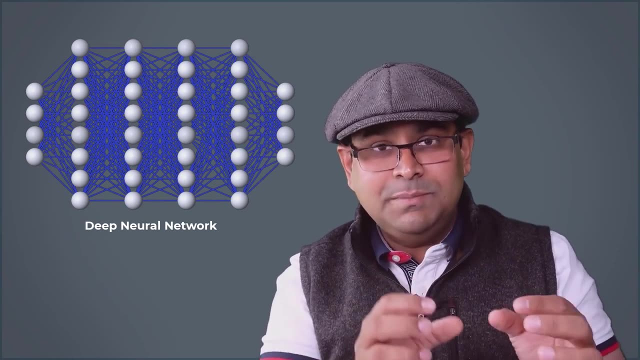 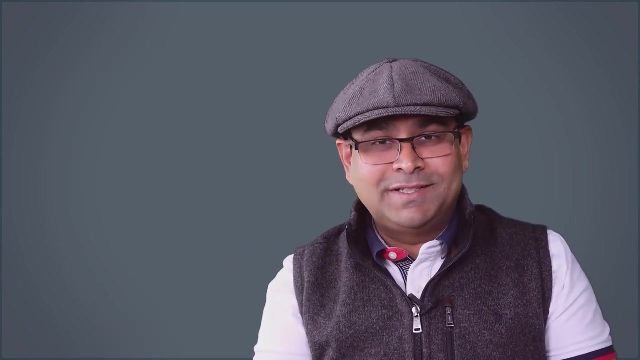 that they could get fantastic results if they trained neural networks with many hidden layers, And this architecture was called deep neural networks. The deep stands for the many hidden layers in the network. But neural networks had become uncool, They were very unpopular, and so it needed rebranding. 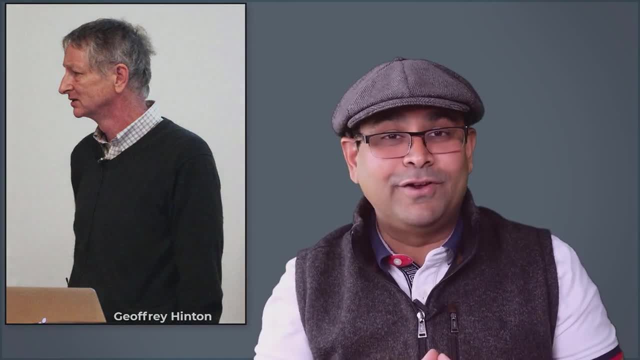 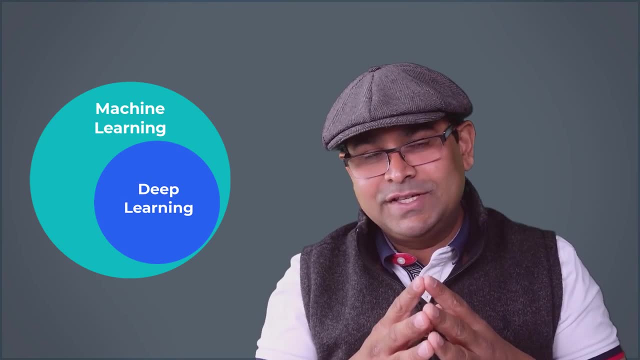 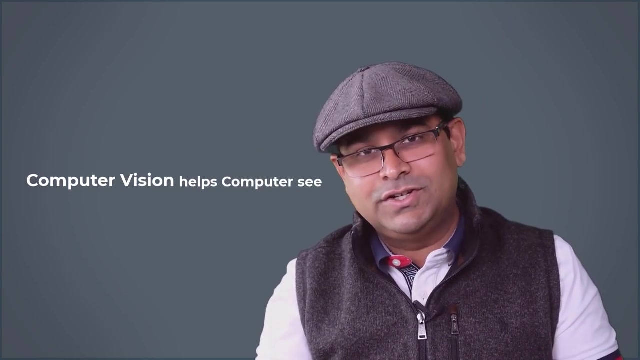 In 2006,, Dr Geoffrey Hinton coined the phrase deep learning. Now that is cool. So deep learning is a subset of machine learning, where problems are solved using deep neural networks. Now what's computer vision? Roughly speaking, it is the field of research and development. 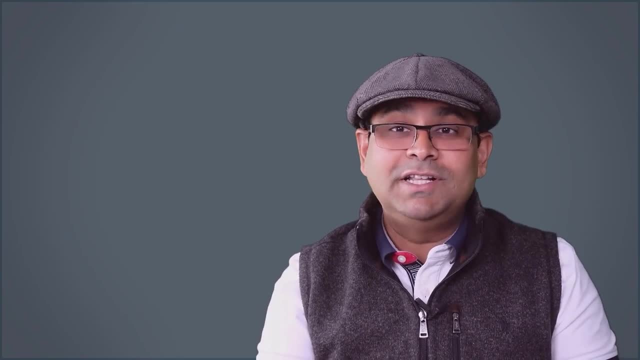 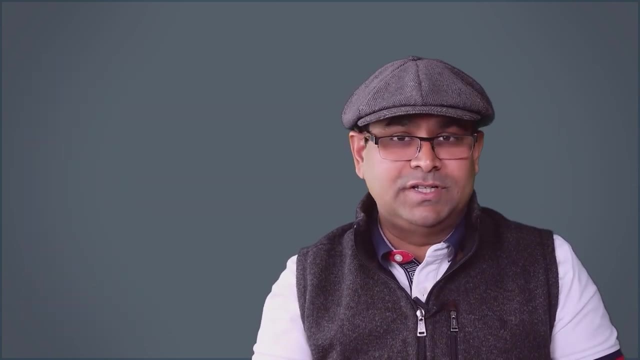 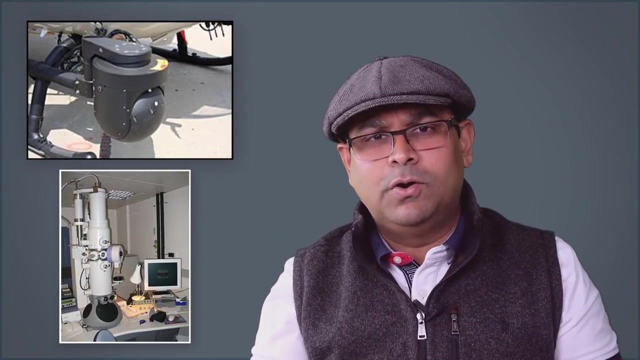 that helps computers see. Computer vision deals with interpreting visual data like images and videos. These images could be from different sources, like computer vision, computer vision with a computer vision camera, a depth camera, a thermal camera, an electron microscope or an X-ray machine, a radio telescope and many more Within computer vision we solve. 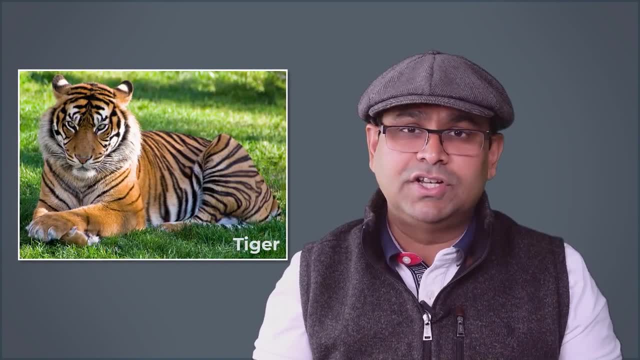 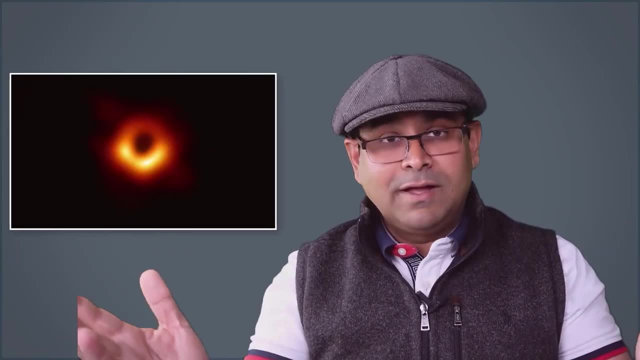 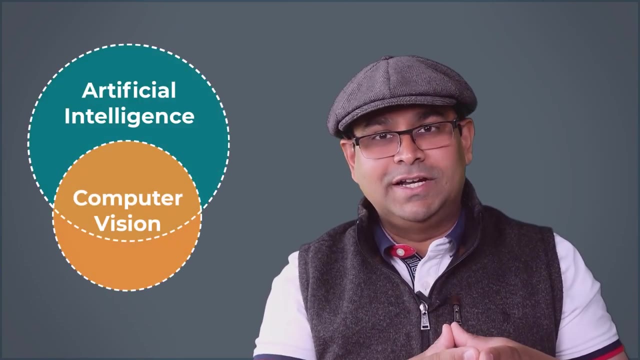 many problems like face recognition, image classification, object detection, text detection and recognition, 3D reconstruction of scenes, photographing a black hole- yeah, that too intelligence, but they have a huge overlap. Many problems in computer vision are solved. 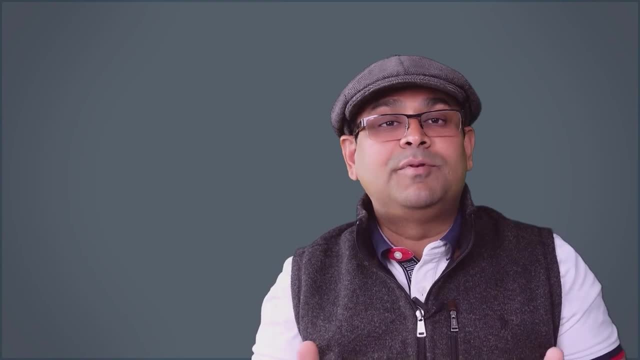 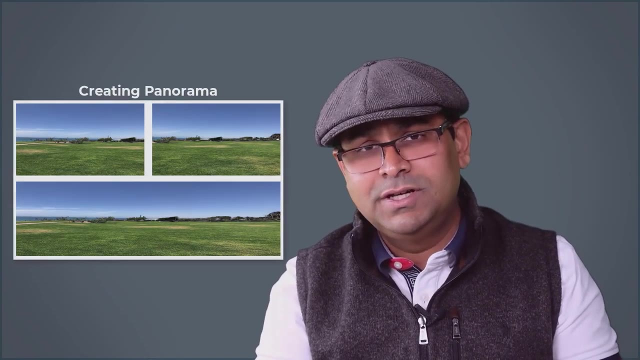 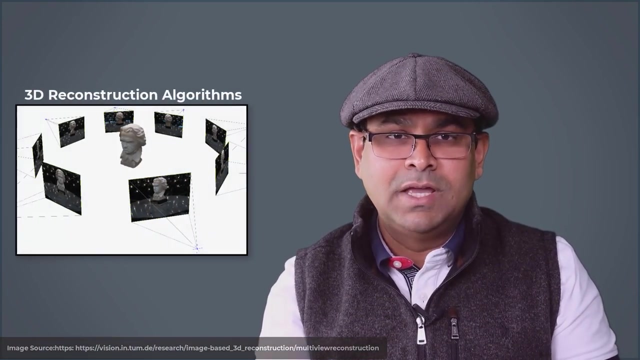 using machine learning, including deep learning, but many other problems are solved without any AI techniques. For example, creating a panorama is part of computer vision, but it usually does not involve any AI. The same is true about 3D reconstruction algorithms. 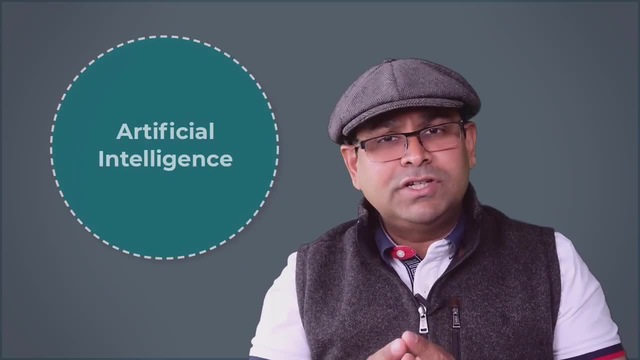 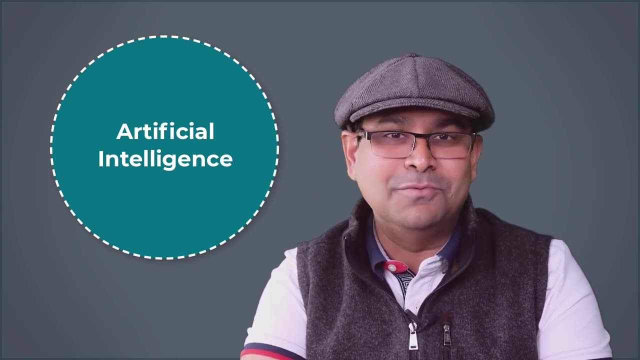 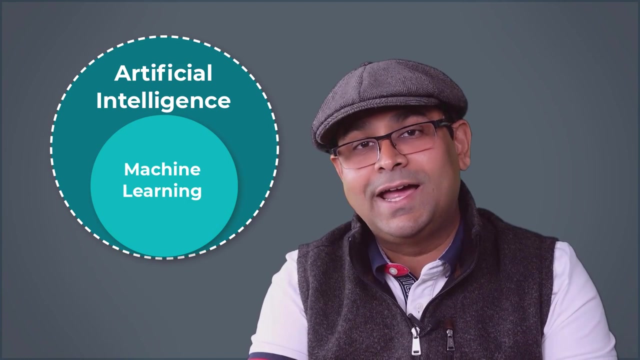 So now let's summarize what we have learned. Artificial intelligence, or AI, is the science and engineering of making machines learn, think and act like humans. Machine learning is a subset of AI where machines learn directly from data instead of hand-coded rules. Deep 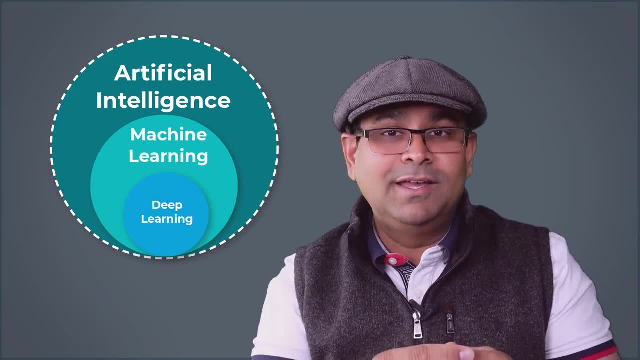 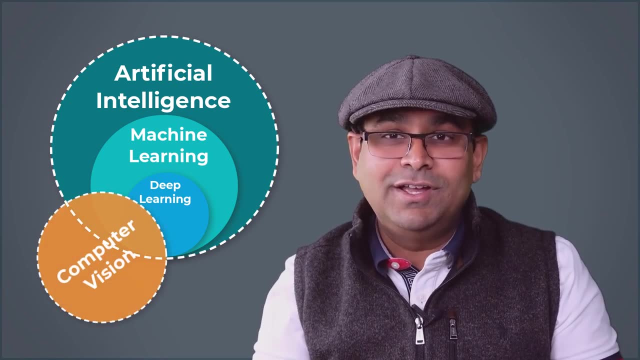 learning is a subfield of machine learning where machines learn using deep neural networks. And finally, computer vision is the science and engineering of interpreting visual data. Many computer vision problems are solved using AI, But many tires will eventually become impenetrable machines. But the most important thing about 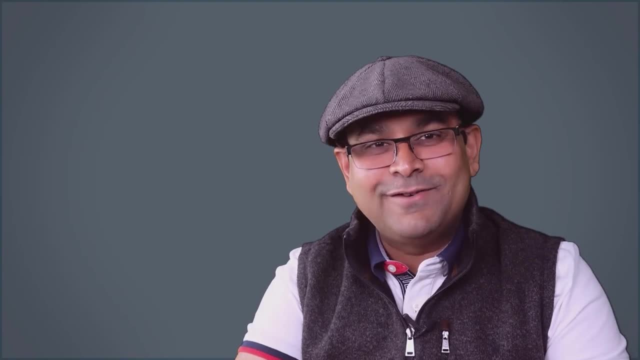 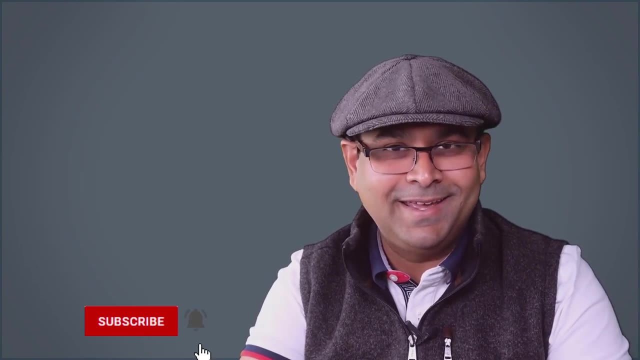 AI is the design and maintenance, Because AI has upstairs and the workup to actually others are not. That's all, friends. If you liked this video, please subscribe to our channel and don't forget to turn on notification by hitting the bell icon. 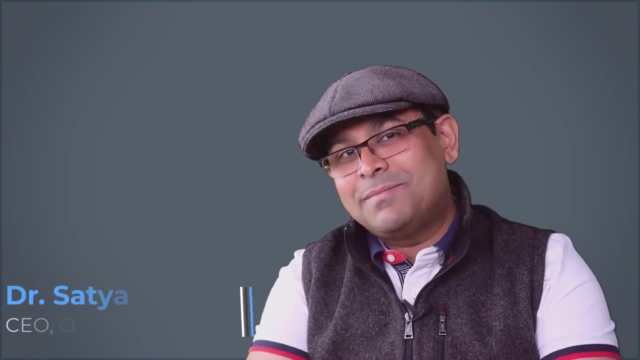 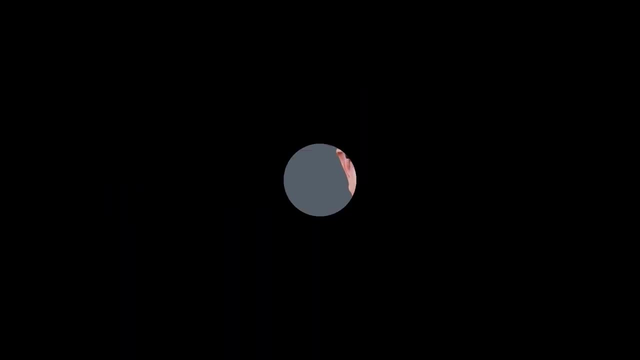 We'll see you in the next video. This is Satyamalik signing off your guide to the fascinating world of computer vision and AI. Thank you.